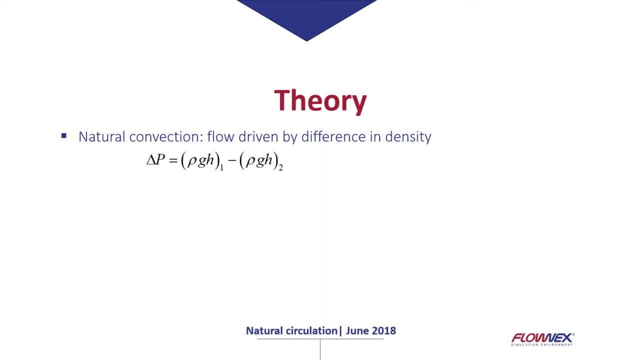 position, minus rho gh on the other position. So the difference in rho gh between two positions will then cause flow to occur. We can see from this that are density is obviously a main driver and then the height as well, Difference in density Cast by difference in temperature. Obviously, if we're working, with a gas, then the higher pressure or change in pressure will genre merk the temperature. So this is the level of density, which神 and fury the method of transformation. Imagine that you've got steamЗдo, you're adding pressure, and then�nm, вмž. you're adding water up, You are entering a Saralsyu developer, what I now call the. 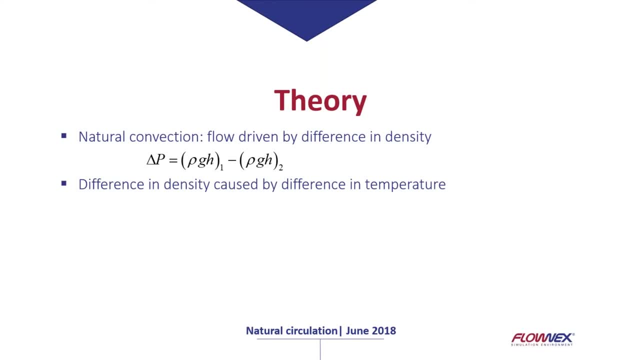 also change our density, but in this case, where we are working in the scenario and working towards reactive reactors, natural circulation- the main, the main factor or the main driver of density difference is caused by temperature. so we'll be focusing on that modeling detail that is required or else stated. 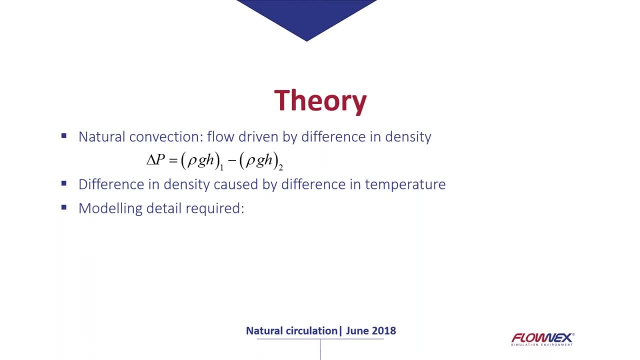 the factors that determines our the amount of natural circulation will be the temperature dependent density in the fluid model. okay, so let's stop there. I've had some examples in the past- and actually I've tried that myself- to have a reactor where I'm working with molten salt and in Flonix I've generated a. 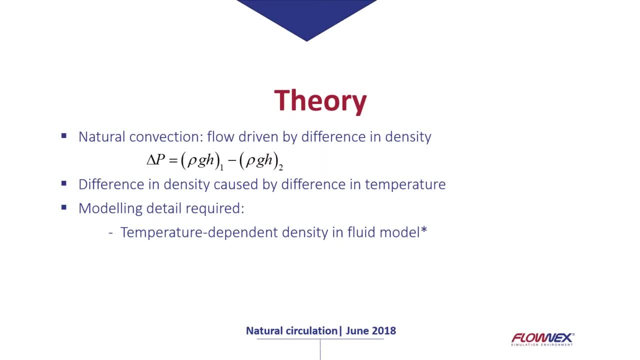 fluid that had a constant density, and I tried to get my network going for natural circulation and I simply could not get anything right. and then, after quite a long time of struggling through it, I realized that it will never work. for in order to model natural convection we need to have a temperature dependent fluid. so in Flonix you'll need 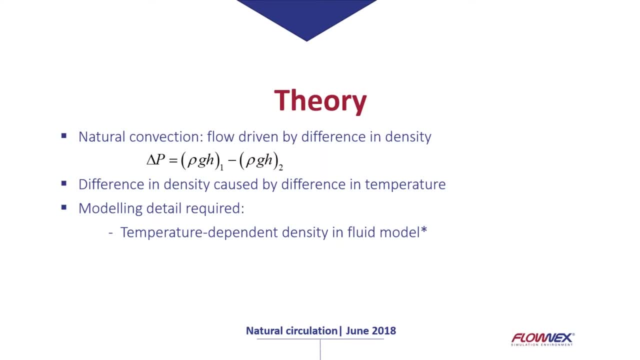 to go into your charts and lookup tables and where you define your fluid, make sure that it changes with temperature. your density now it changes with temperature. that is extremely important. also, we need some, some elevation specification. if all your pipes are in a flat line in the horizontal line, we're going to have some difficulty getting. 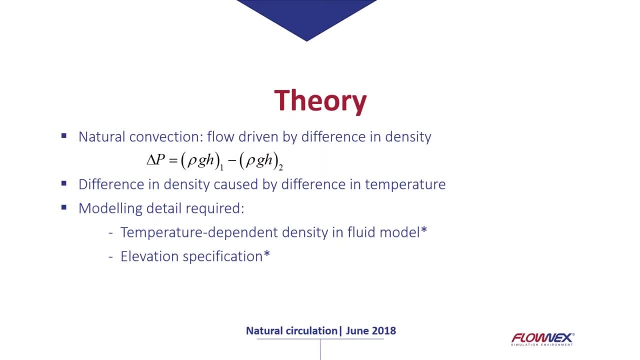 that natural circulation going. so obviously we need our elevation specification as well, which is very important. and then, lastly, heat transfer: we need something to create that change in temperature in order to have the natural convection flow in the end. so those three parameters, or those three factors, scared a thing: density: density supply after high-end C. 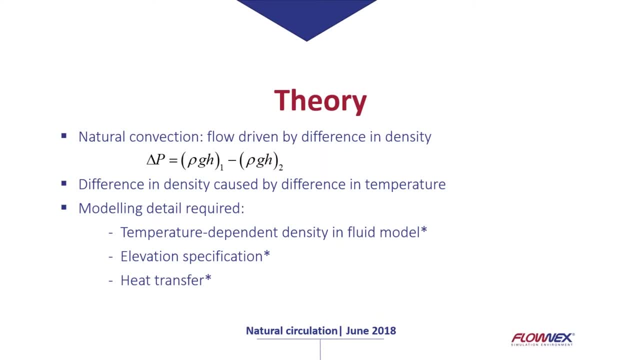 Is so those three parameters are for if in a numerical process the temperature dependent density check. the W prediction code I have placed as it straight in this picture: in the fluid model, elevation specification and then heat transfer. addition is imperative in order to get natural convection going. 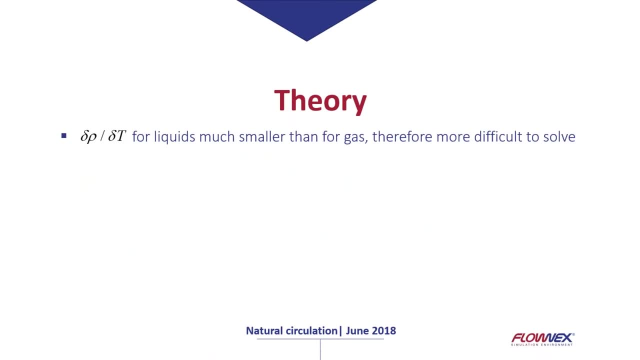 just a note, something important to understand the change in density with regards to the change in temperature for liquids are much smaller than for gas and therefore it is more difficult numerically to solve. so what we are talking about, if you think about the, if you have a pocket of air, 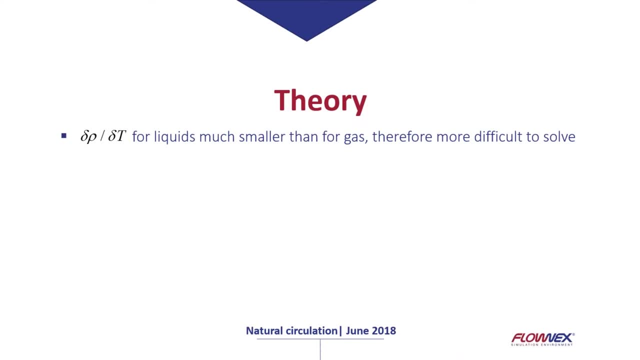 or a pipe of air. with just a little bit of heat you can have quite a large change in temperature and with that then have a large change in density or a large enough change in density with water. on the other hand, you need quite a lot of heat to have a significant change of temperature and even 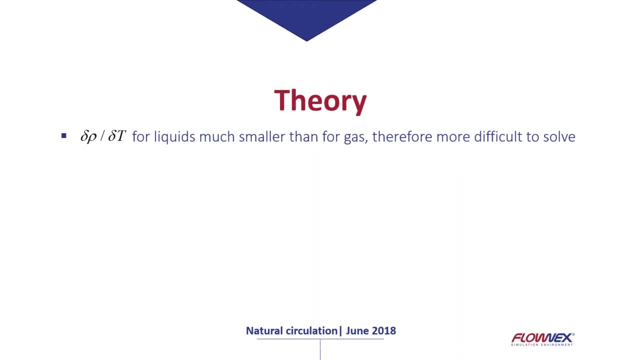 with that significant change of temperature, the change in density will not be that much. so it is a lot easier to get natural circulation or natural convection with with gases than it is with liquids or with molten salts, so keep that in mind. if we are working with a network then we should apply temperature gas values and even work with 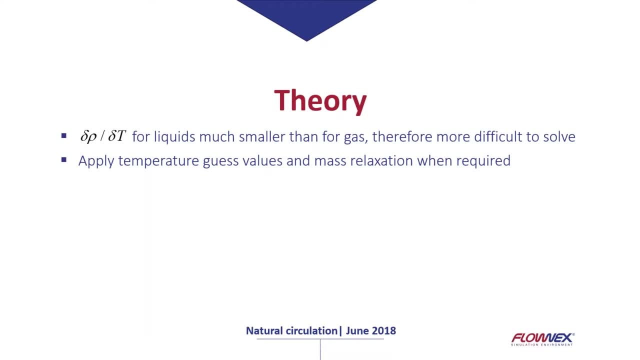 mass relaxation when required and during our session where we were going to work with flonix, i'll give a quick discussion and overview of the flow. next i'll give a quick discussion and overview on that. and then, lastly, ensure grid independence with component increments. so when 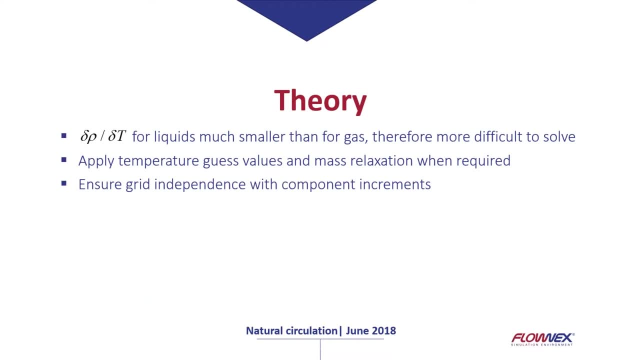 you're working with your pipes, make sure that you have enough increments so that you capture all your data. try to increase your increments and see if your results change significantly. if it does, then you know you have not yet reached grid independence. let's quickly look at this youtube. okay, so we have a tube here. 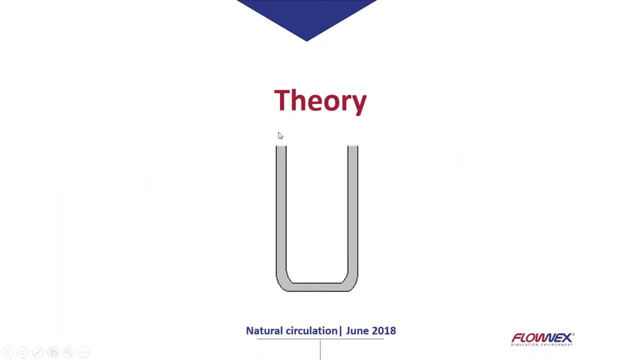 and currently i can just get my arrow going there. so it's filled with some type of fluid. whether it's gas or water or liquid, for now it doesn't matter. so it's filled with some type of liquid and currently we don't have any flow. say, for example, we add heat now on the right hand side. 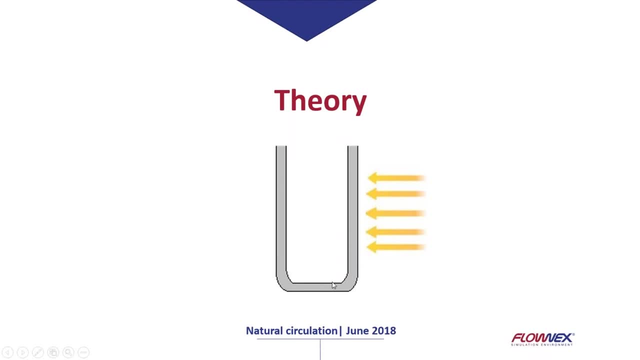 okay, so i need you to think about this before we go on. my question will be: will we have flow in a counterclockwise direction or in a clockwise direction? okay, so just think about this for a moment. intuitively, my mind tells me that, since the heat is added on the right hand side, 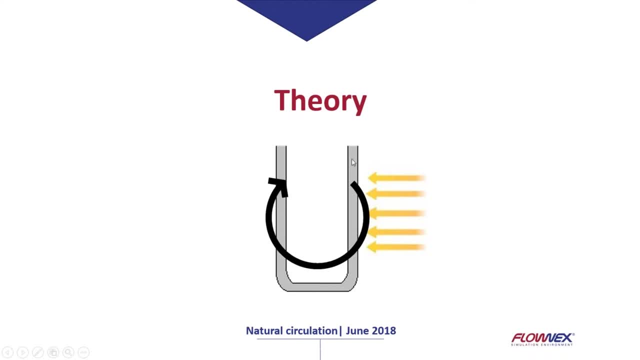 that my column will, or my movement of fluid will go counterclockwise, so it will heat up and therefore will end up in this tube. so immediately the flow 씨up in this tube and go outwards. that's what my and flow outwards. that's what my mind tells me. however, that may not be the case. 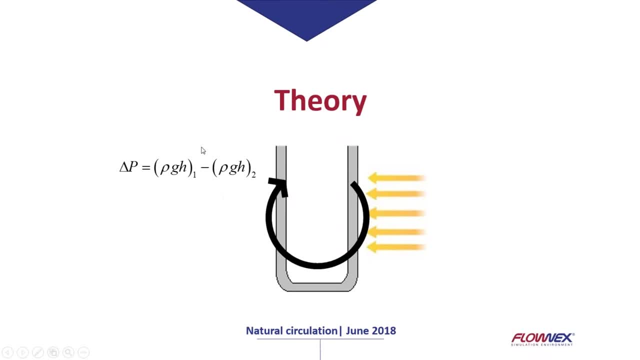 in all circumstances. if we look at the equation again for our flow driver, so delta p equals the difference in rho g h say. for instance, at the beginning i had some flow going in a counterclockwise in a counterclockwise direction- sorry, in a clockwise direction- and so i need flow in a clockwise direction. 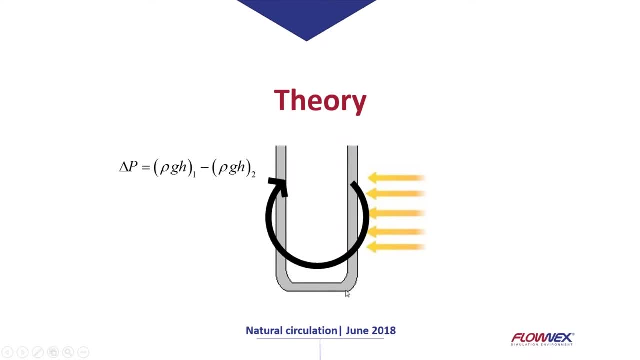 going here and i add my heat. it means that the density in this tube here will be less than the density in my right hand tube. so you can think of it as the weight in my right hand tube will be more than the weight in my left hand tube and therefore i will actually get. 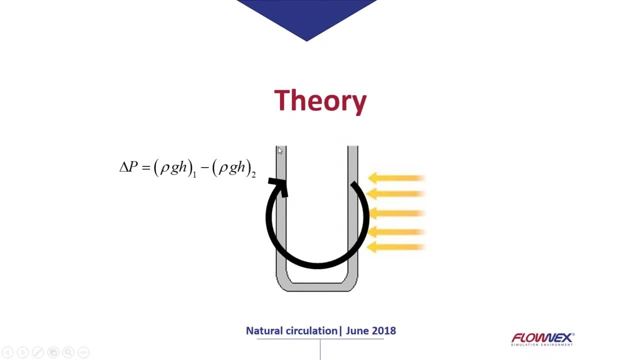 flow going in a clockwise direction. so, thinking of this, you can see that natural circulation is quite an intricate and finely balanced flow phenomena so i can have them in both directions. both directions are feasible or in realistic, in real life are possible. so something needs to, needs to start that process, something needs. 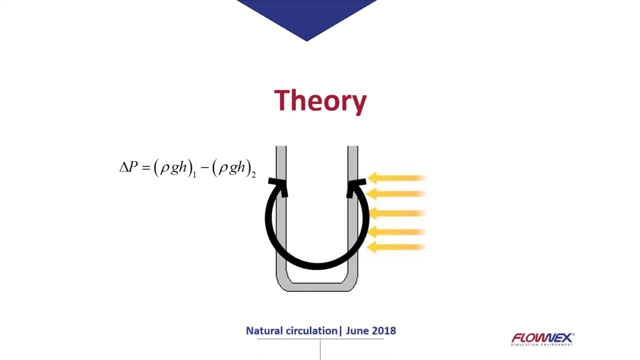 to start that process, something needs to give direction to my flow and then, afterwards, give direction to my flow and then, afterwards, the change in density will maintain or increase. the change in density will maintain or increase that flow. but in order to get that flow going in that flow, but in order to get that flow going in one or the other direction, there needs to be some. 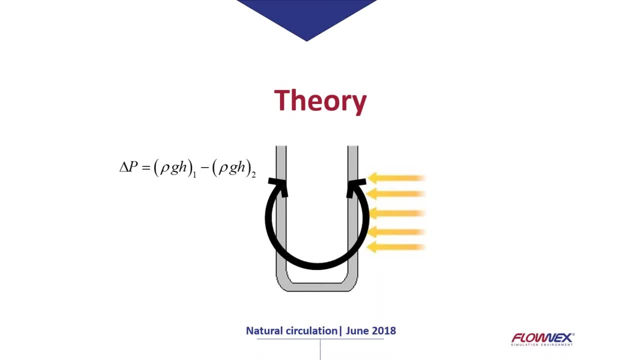 some, some starter to that, if i can call it in that way. so it is important to understand that natural convection in this case can go both ways. if i have a youtube and i'll show that to you as well in the flow next network. last comment on this, it is important to keep in mind the pressure. 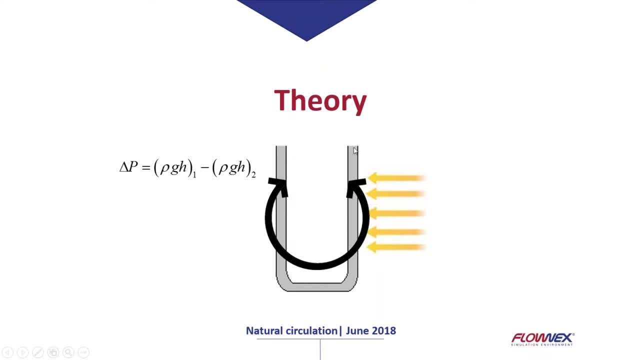 on the inlet and the outlet of these tubes. now remember, not everywhere the, the, the ambient pressure. the ambient pressure is not the same everywhere. i mean even between the first floor of a building and the third floor of the building, there is a change in pressure. so at sea level we 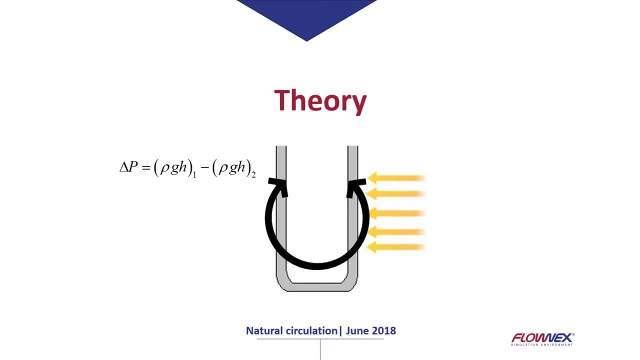 might have say, for instance, 100 kpas or 101 kpa of pressure, but as i go higher that pressure decreases, my ambient pressure decrease and that will have an effect even with one meter of change in height. that will have an effect on my boundary condition pressure on the inlet and outlet. so if 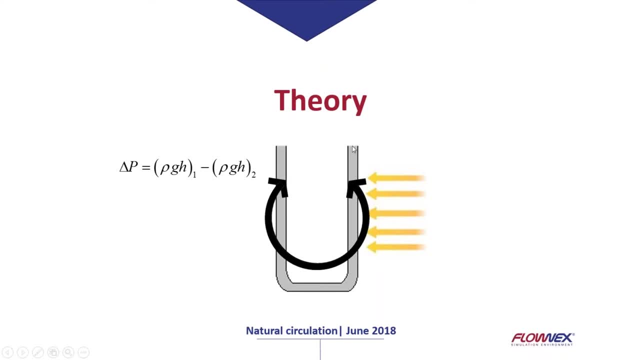 i have different hydraulic heights on the inlet and outlet. i need to precisely account for that in my model. and then, lastly, in order to get it going into a certain direction. so say, for instance, i know that my flow will be going in a counterclockwise direction- i need to add guess values to 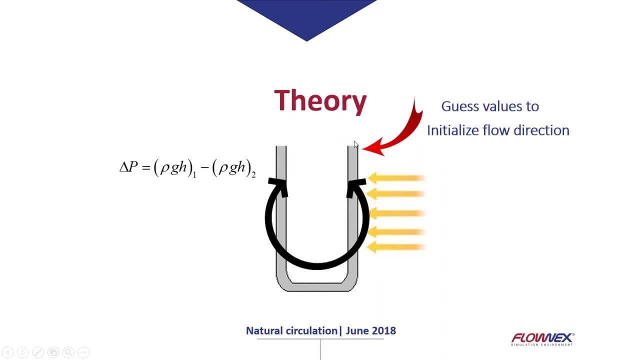 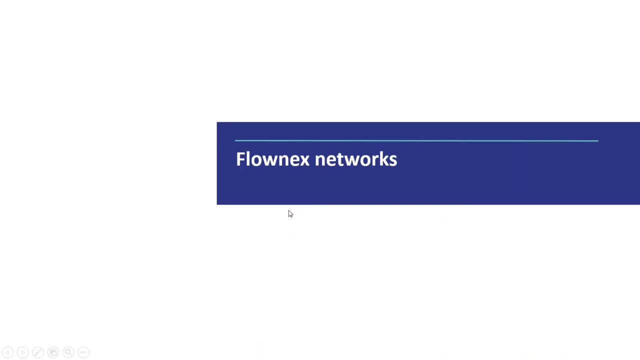 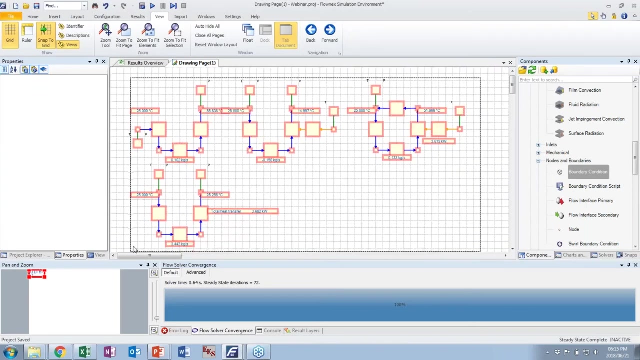 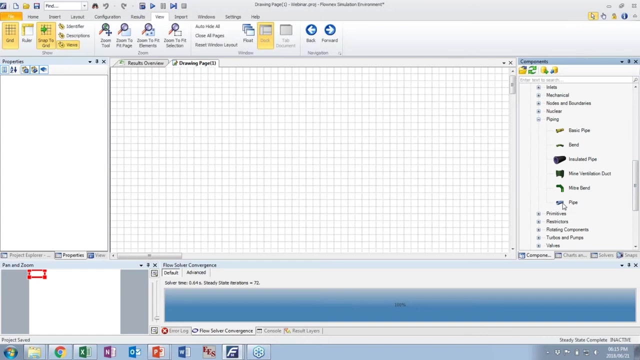 initialize flow in that certain direction, and i'll show you how to do that in just a minute. so let's go on to our flow. next, networks: just going. okay, i'll be cleaning all my previous exercises and start the fresh, okay, so let's set up a youtube example, so the one that we've just discussed. 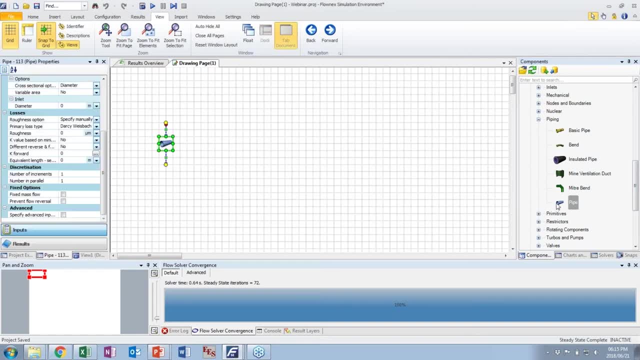 um, let's get our pipes in there, so that will be the downcomer pipe. i'll add another pipe on the bottom and then the pipe, the riser pipe again, i can select all three of them and give them a length of 10 meters. let's say a diameter of 0.3, roughness of 100, and let's give it 10 increments to start. 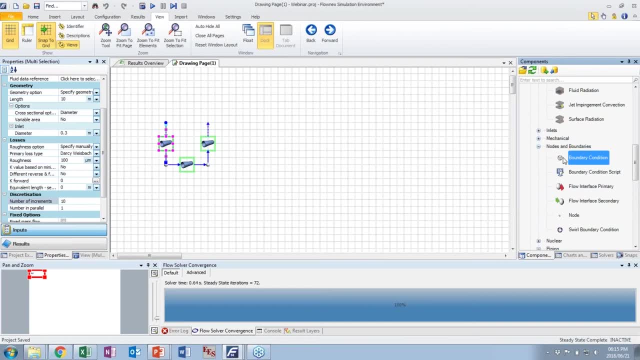 off with. i'll add my boundary values to the inlet and the outlet or to the various ends. let's say both of them are at the same height, so they will have the same pressure. let's say 100 kpa and this one, which i assume to be on my inlet, will have a temperature of 25 degrees c. 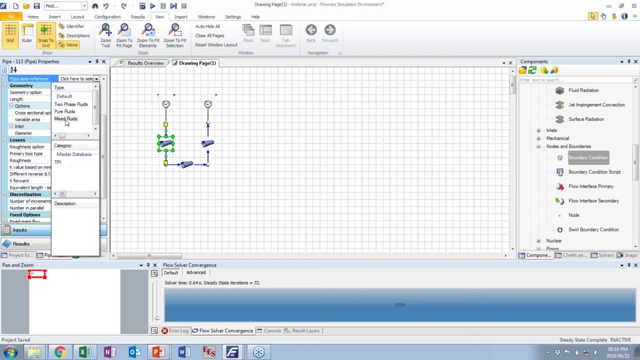 i need to add a fluid specification, say, for now we are working with air. and then, lastly, i need to add my elevations on my node, so i can click on both nodes together and then say they are 10 meters at height. so these two are zero meters in reference, and these two are 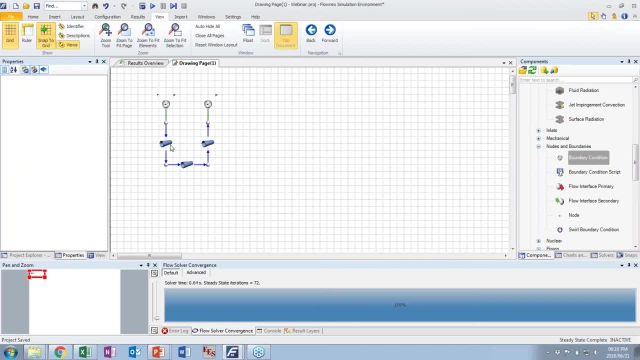 10 meters um. lastly, now let's get my results going. so i would like to see my total temperature results there on that side, and then also my total temperature results on this side, and then my mass flow. i would like to see where my flow is going. total mass flow. 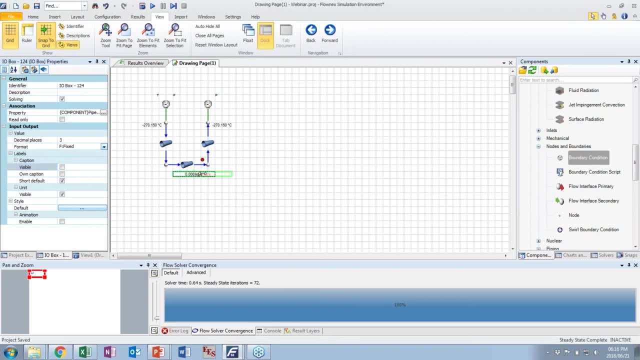 all right, let's solve it and see what happens. okay, brilliant, i have a converged solution now. at this stage, i would like to point something out. since i've been working on in this project previously, i've already changed my mass relaxation, as i mentioned previously. uh, in the network or in the presentation it looked strange, but it makes thirty percent. 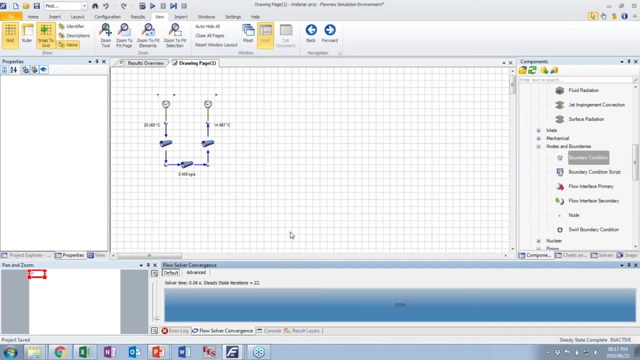 better it. Hamid Siddiqui boarded up for me. now let me show you what's most characteristic of it. sorry, i'd say nothing, but it makes things better. sometimes it may be necessary to have mass relaxation. I would quickly like to show that to you, so I'll go to solvers. you're on the right hand side of my. 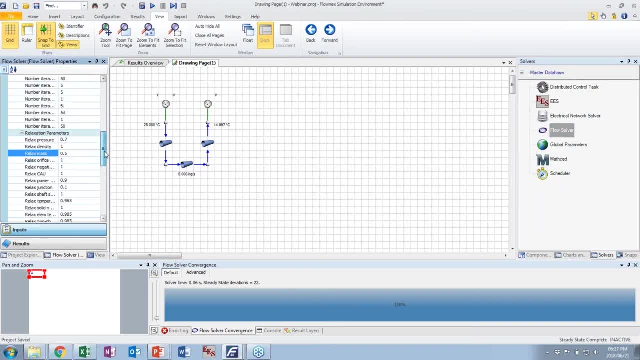 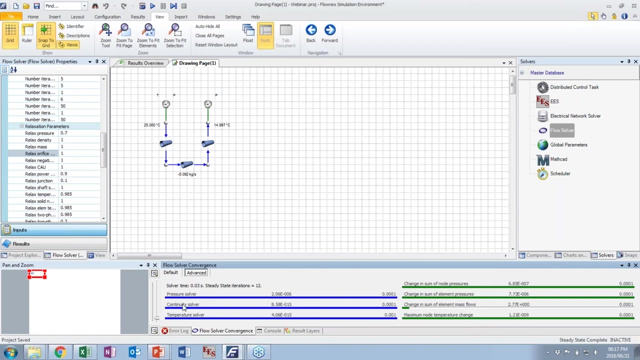 screen. click on flow solver, go to mass relaxation. by default this value is normally one and now if I solve it, I will see that I don't achieve full convergence. in this case, if I click on my advanced flow solver convergence button, I'll see that all my or my pressure solvent, continuity solvent. 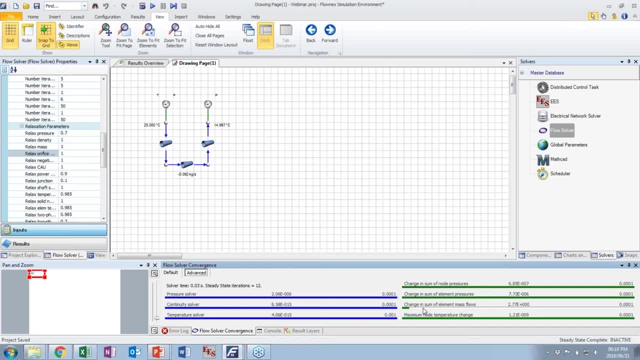 temperature solver. all these converged fully but my change in sum of element mass flows are still lacking a bit. so this gives me a clue as to the fact that I have some difficulty solving the mass distribution, the mass flow distribution, through my system, and with that then I can go and change my relax mass to let's. 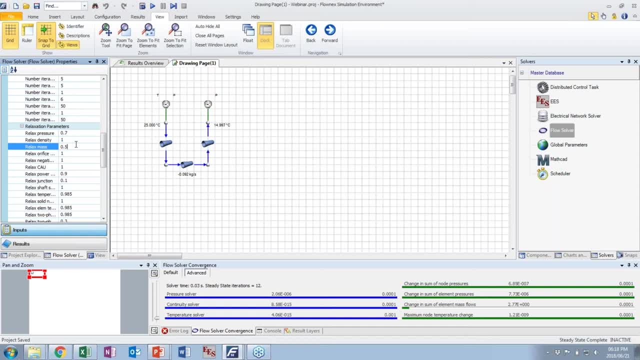 say zero, point zero and five or whatever value is needed. I would like to stress that please don't go and play with your relaxation parameters each time. you don't get convergence only if you're a hundred percent sure and you understand the complexity of your network and the mathematics behind that and you know. 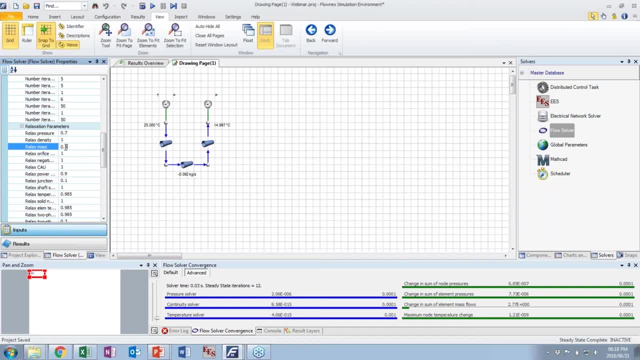 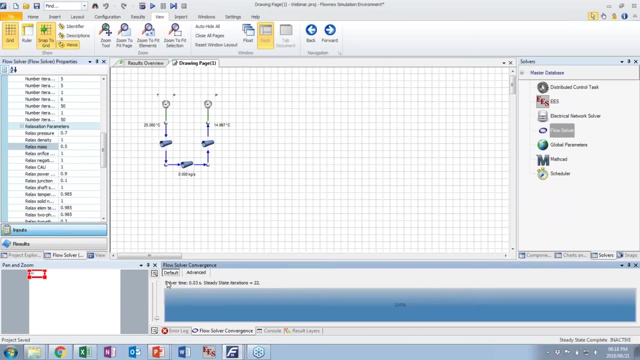 that you should be working with these values, then you can go to that. so just just a reminder they- this is only a last resort. if you are a hundred percent sure that your network has been set up, perfectly, okay, and now, if I solve it, I'll see that I obtain full convergence in the default window. I can say I have. 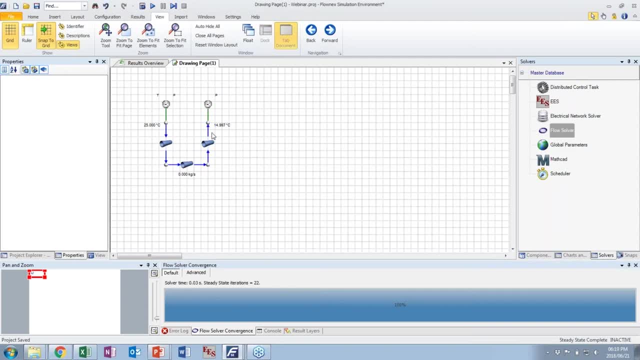 hundred percent values. next thing that I want to point out is the fact that I have no flow. I can see there's no flow through my system. remember, we didn't add heat yet, so this is just a normal YouTube configuration without any heat, but the temperature on this node here is 15 degrees C. the reason for that is that 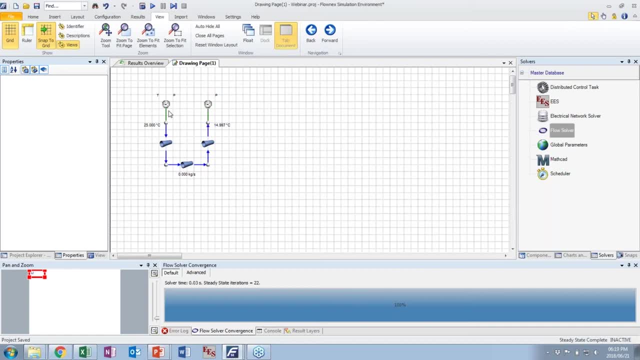 since I have no flow, there's no cause in flow next to get this temperature of 25 degrees C through my system and to move it up until this point. so that's 15 degrees C is my default ambient value, which also is specified in my flow. 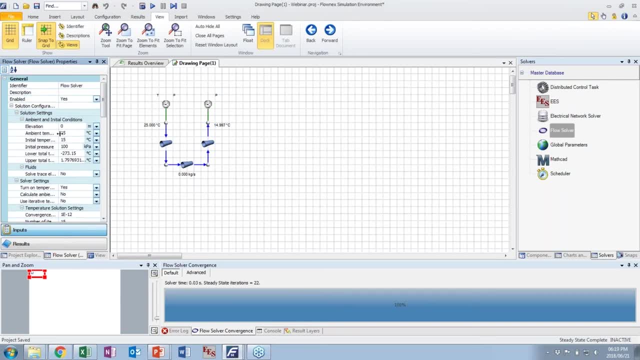 solver and go to the top, my ambient temperature default value. there is 15 degrees C and that is where that 15 degrees comes from. so since there is no flow, there's no movements of fluid in my pipeline, Flonix will assume that 15 degrees C on these points and then, obviously, my 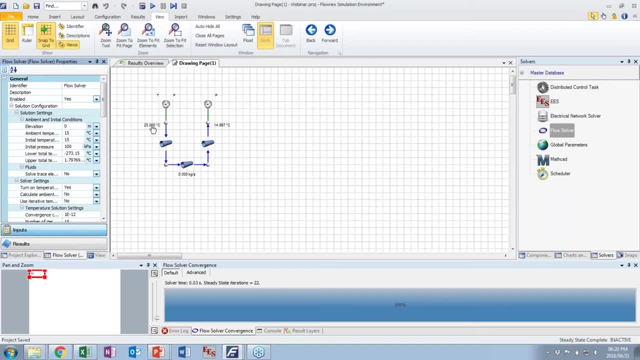 boundary value, where I specified my 25. that is where this temperature comes from, right. next step is to add heat. so let's go to this pipe, go to the input. I would like to specify advanced input code. this is where I add my heat. so, advanced input. and let's start off with a fixed exit temperature. so by. 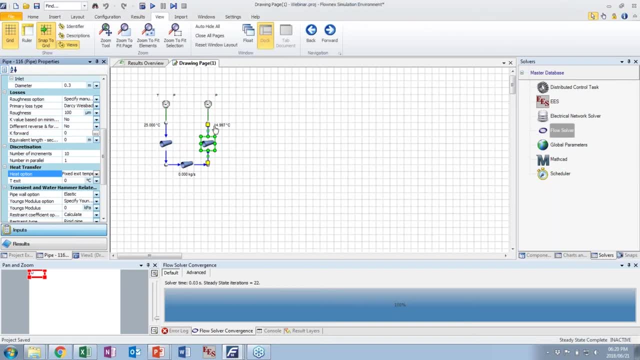 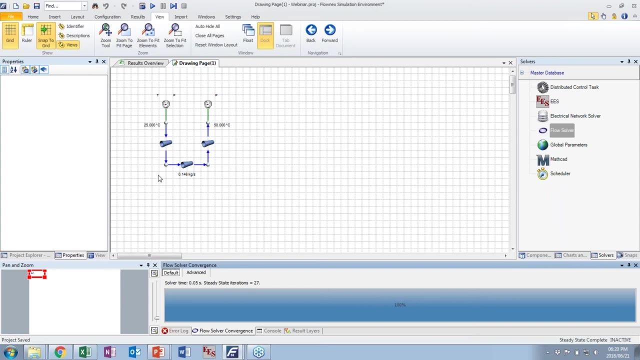 specifying this, Flonix will make sure that the temperature and the outlet of this pipe is 50 degrees C, and it will calculate what heat needs to be added in order to achieve that. so let's say fifty degrees, and now I can solve it. ok, great. 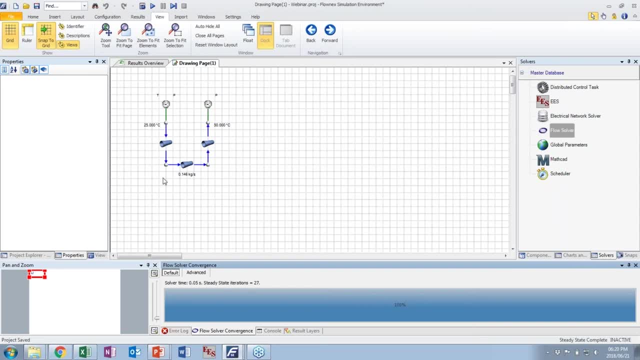 it goes in the in my, in the right direction which I wanted it to go in from, from 25 degrees up to 50 degrees c, and let's see how much heat was added. so i can go to my results: total heat transfer, and it is just over a tad over three and a half kilowatt which is required. 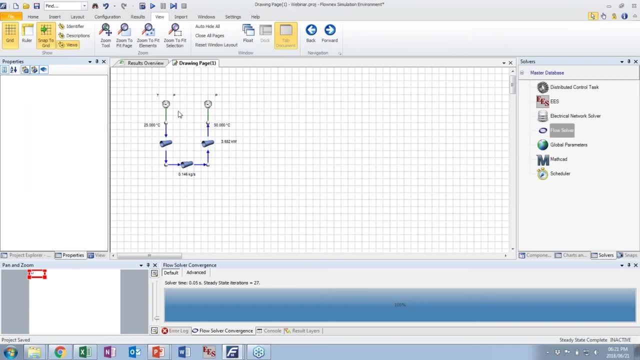 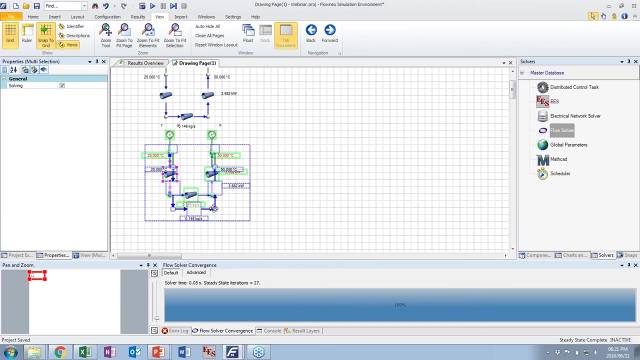 to get this flow of 0.146 by means of natural circulation, from 25 degrees c to 50 degrees c. okay, this is a simple example. with air, i can also copy this network. let's say copy and then paste it here. i would like to show you an example with molten salt. so i'm going to change. 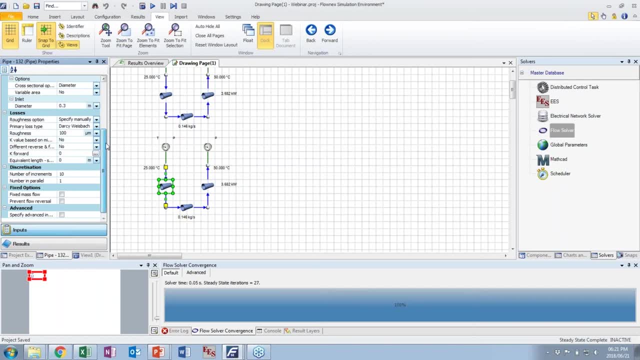 the fluid to molten salt which i've changed, generated previously. so i'll go to molten salts and my hdrx molten salt and now i can solve it again and due to the change in temperature from 25 degrees to 50 degrees c, i need 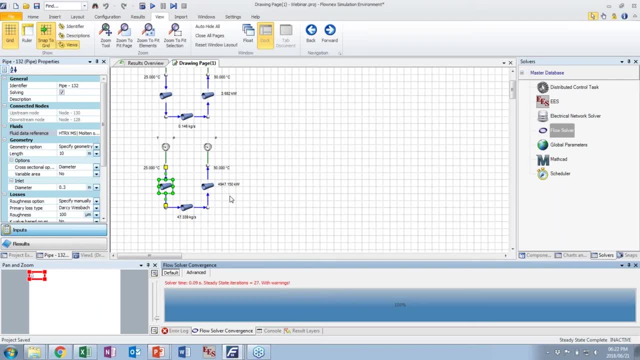 almost 5 000 kilowatts, or 5 megawatts if my maths are correct, and then that change in temperature will cause almost 50 kilograms per second of this molten salt flowing through my system, and then i can go to the next step, which is to change the temperature of this molten salt. 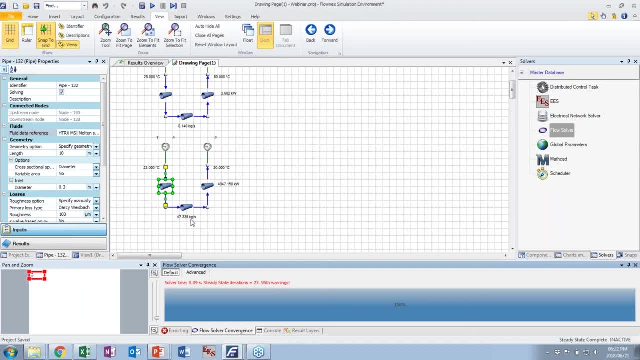 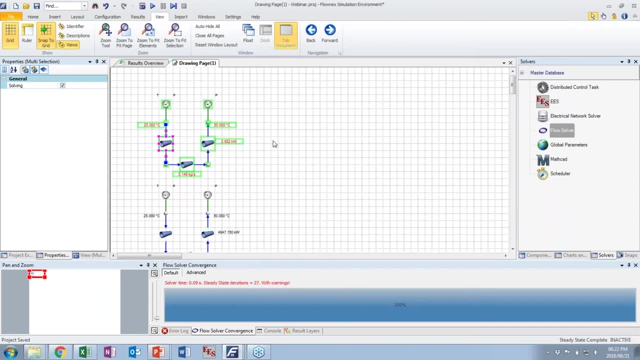 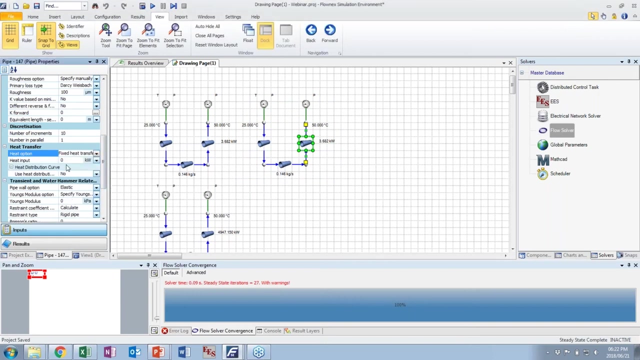 system purely due to natural circulation. another example which we might do: copy this again. i'll paste it here alongside this network. so another way of adding heat would be, instead of specifying my fixed exit temperature, i can say fixed heat transfer and let's go for more or less. 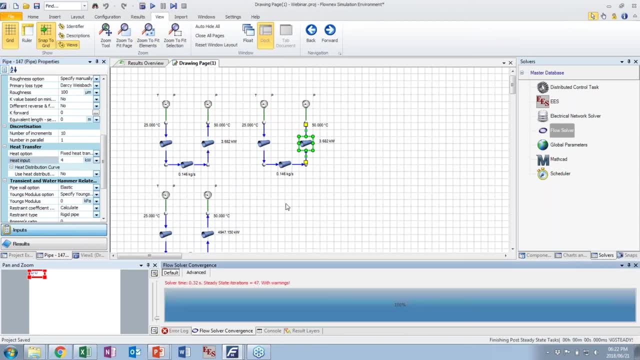 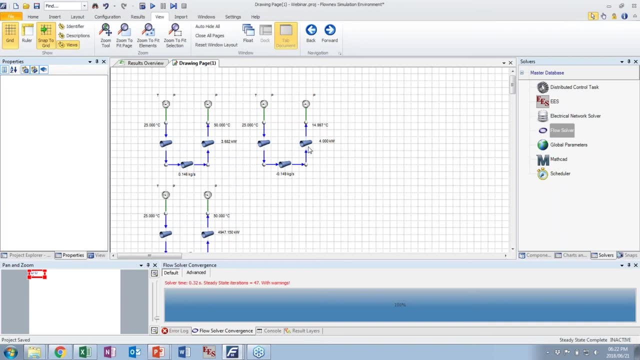 four kilowatts and see where. we see where we end up. all right, this is brilliant. so just to see the difference, i've added four kilowatts of heat here. now the amount of heat doesn't matter, it's just that, due to the way in which flonix was, 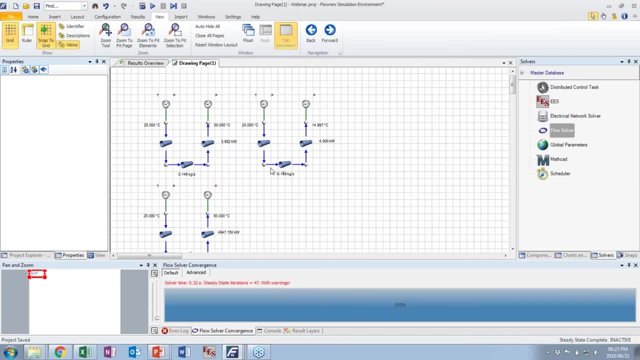 initialized. in this case, i got flow in a clockwise direction. now, as i've explained previously, this is not wrong in any way. this is exactly what can happen in reality and since, since there are no there's no history in terms of flow direction, it is perfectly possible for flow to come this way around, so it will. 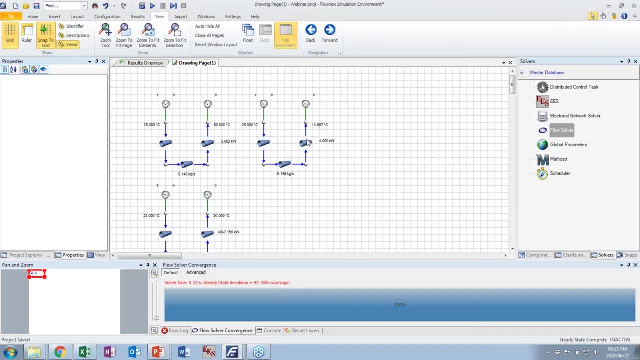 come in at my 15 degrees c, it will pick up four kilowatts of heat and my temperature here that you can see on the flag, 41.7619 degrees c and then, obviously, due to the fact that i've in four this temperature here on the boundary value, it will go back to 25 degrees. 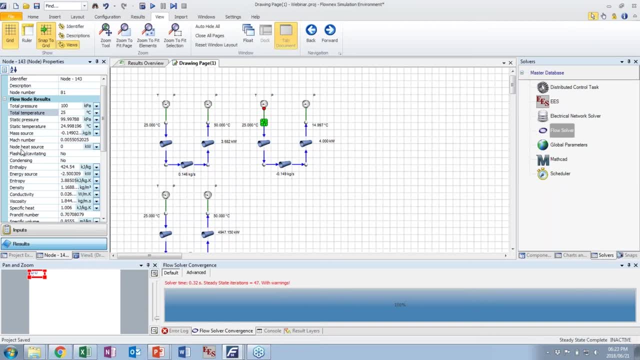 with an energy source. there's my energy source. okay, in order to get it back into a counterclockwise direction, what i need to do is to help flonix initialize its flow in the counterclockwise direction, and to do that, i'll click on the node and i'll go to specify. 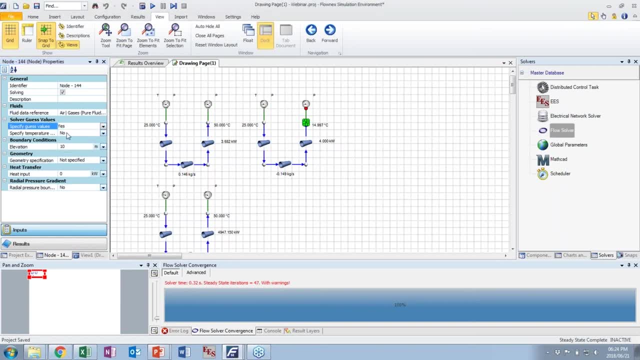 gas values. so i'll change that to yes and then i'll take my temperature gas value and let's say this is more or less 50 degrees c. in this way flonix will start off. it will see that this temperature is 25. this one should be more or less 50. so 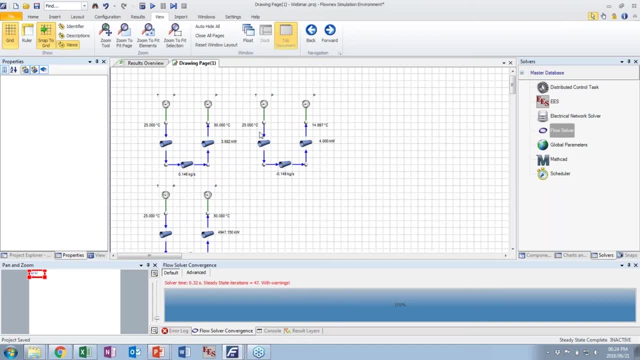 the flow due to natural circulation will be will be driven in this way from each its initialized state and then from there on, it will solve. so let's see what happens. so nothing, am i doing something wrong? ah, there we go. he didn't update, perfect, okay, so you can see now flow going in a counterclockwise direction. 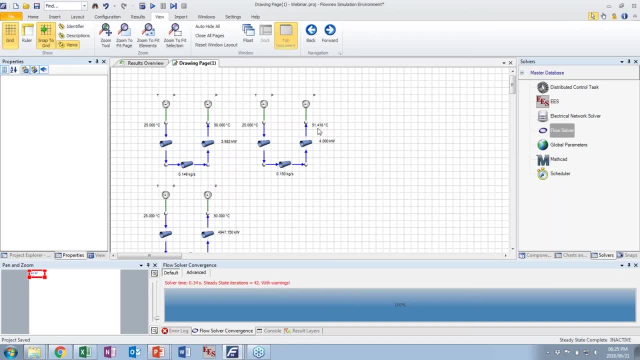 and i achieve a calculated value of 51 comma 418 degrees c due to my four kilowatts of heat added. last example to add heat again. copy this network and paste it on this side, and this time i would like to add a heat transfer element. so let's delete that. 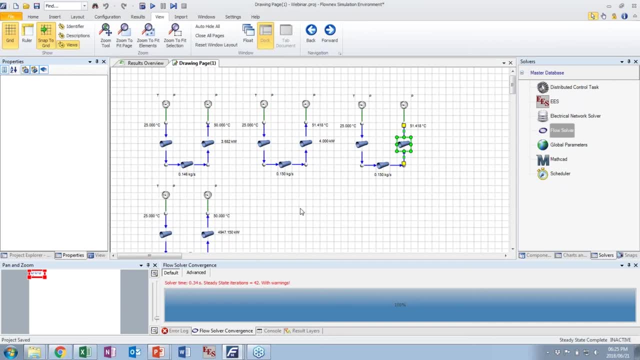 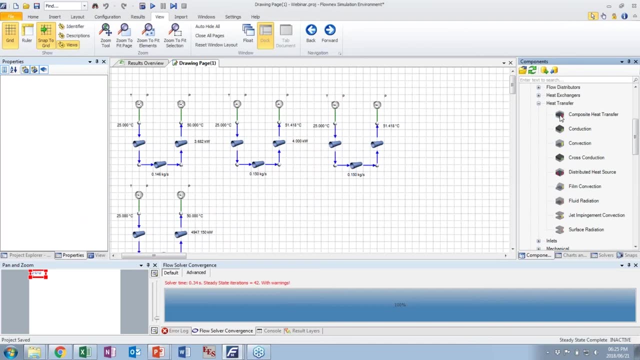 and i'll put this back to zero again, so no heat is artificially added and i can go to my components. take under heat transfer my composite heat transfer component and let's add a boundary value. so let's say my minimum temperature is 1 degree. temperature on the outside, on ambient conditions, is 100 degrees C. I'll quickly 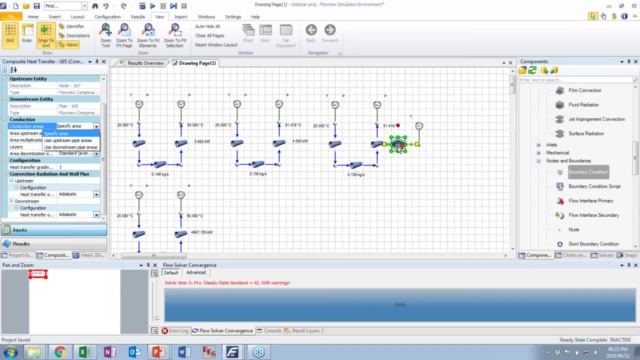 set this up. so my the area, the heat transfer area, can be received from the downstream pipe area. so this is now upstream, downstream, so this pipe area will be picked up. let's add my solid material. so this just signifies the flow part, the fluid part, and this will now be the solid part. so I can quickly say: 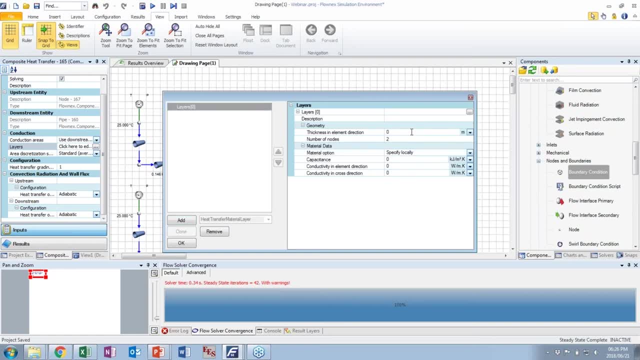 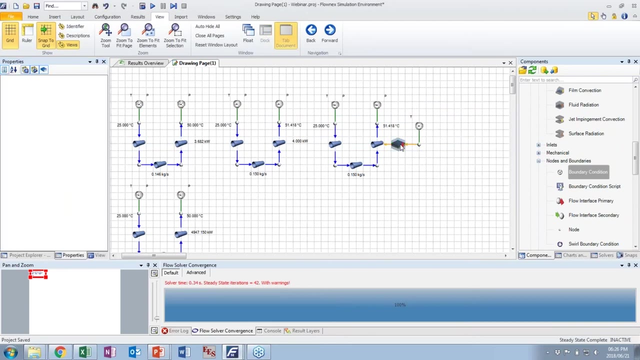 add a layer, let's say this is three millimeters thick, and then select from database. let's quickly assign carbon steel: perfect, from the upstream side. so it's where the arrows comes from. in this case, we can leave it as adiabatic heat transfer and on the downstream side- I downstream side- I would like to add some. 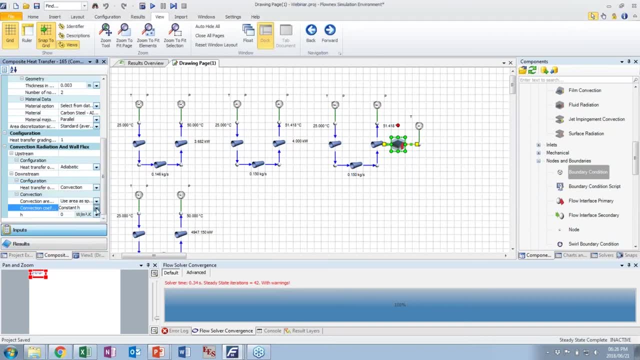 convection and I would like flow next, to calculate the convection coefficient according to the amount of flow that takes place. again, if we solve this- so if I have a pipe that has an else outer temperature of 100 degrees C with the material of carbon steel, then I would realize, or I would 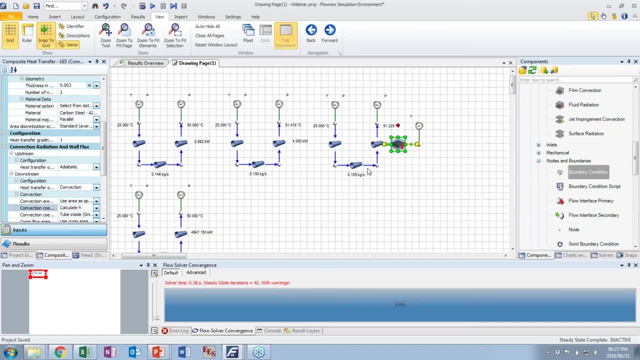 have an effect of a natural circulation in a counterclockwise direction. in this case, if I have a pipe that has an else outer temperature of 100 degrees C, with the Southeast document we would have an effect of a natural circulation using this 효 that creates a unit of zero comma one, five, five kilograms per second. 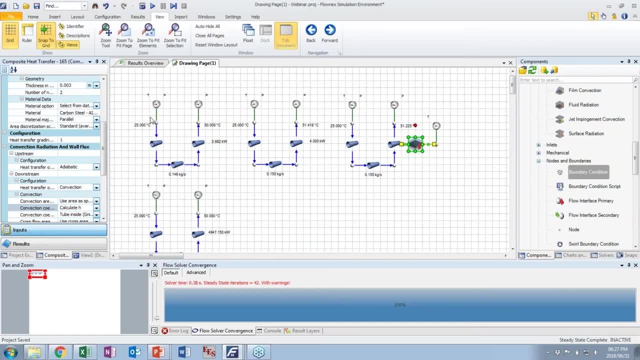 and it would come out at 51 degrees if flesh fluid is air. so there are three examples of how to set up a natural circulation YouTube part in order to see or to visualize my natural circulation flow. the last bit to this is to close my so network. so I'll take this pipe, copy it again as an example, just to show you a closed network, and again moo. so each part contains a unique filter with which I had put another flow to store presence as an example. with this one I am a Marker, again for the reason that this is not a block of a result, that this ط prediction of the flow of the flow has not been solved very most of its points is to check andーno, of course, this is just too quick, so pay close the exclusive expression ofлекс the amount of flow, which is exactly what. 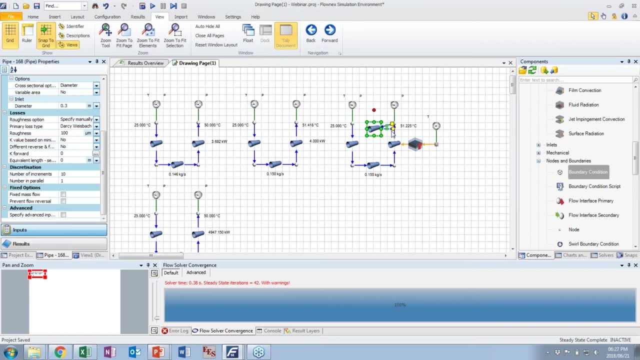 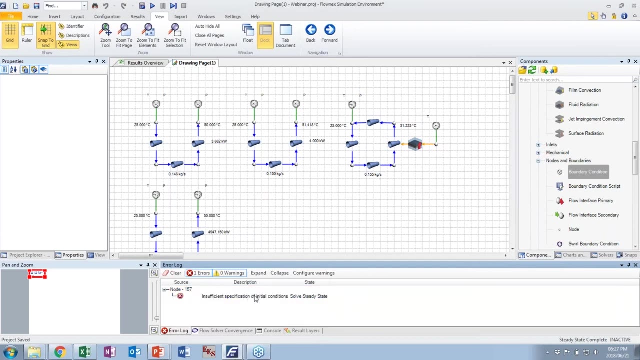 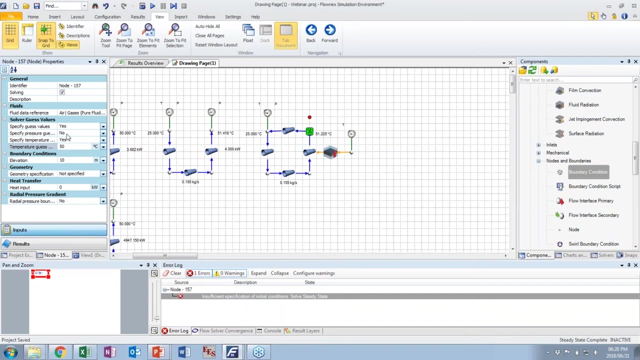 as an example, just to show you a closed network, connect my arrows and now, since i have a closed network, i only need one pressure boundary value and i can solve it again. insufficient specification of initial conditions. i can actually now take my initial conditions off or i can just add a pressure case value. let's take it off and see if it still runs. 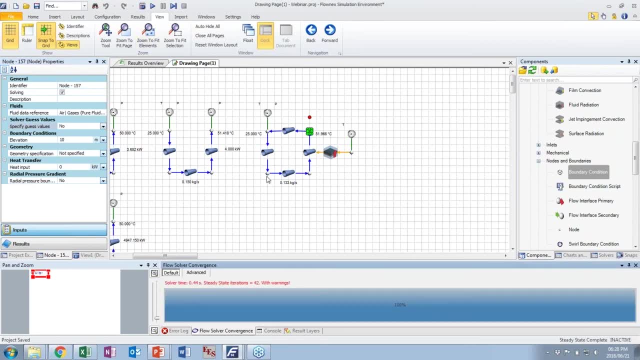 there we go. so there's my network. it's to start off at 25. it will be heated up up onto a temperature of 51 degrees c due to my heat or my temperature added on the outside of my pipe, and then it will come back again and there will be an energy source. 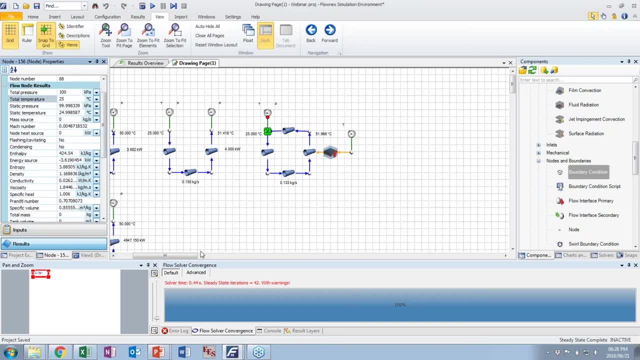 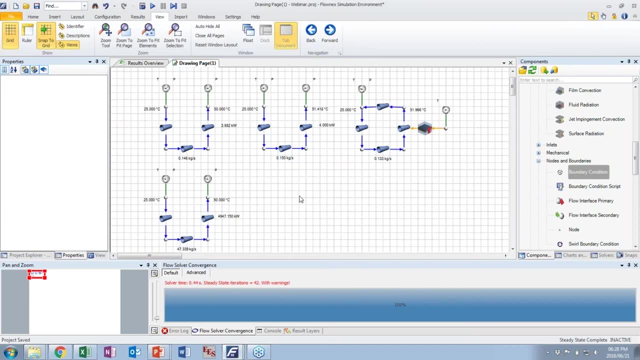 created in order to take that heat out, to take it back to 25 degrees c. and those are the ways, in the simple ways, in how to set up a natural circulation case in flonix. now i spend some time on this. i hopefully i got it to look fairly easy to do this. 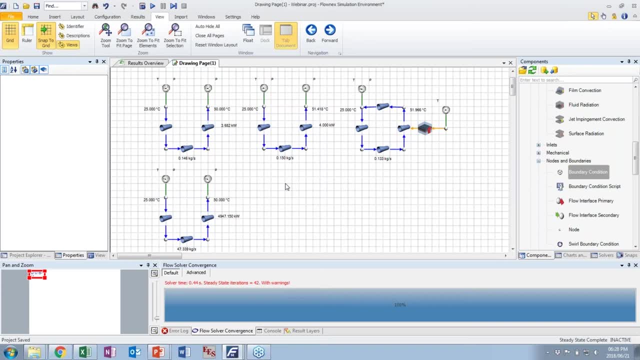 it is not. this is a finely balanced phenomena, again, as i said, and you need to spend some time in order to first of all understand your system and then also get a good feel of how to implement this in flonix. these are very basic examples and you can understand now the moment we take. 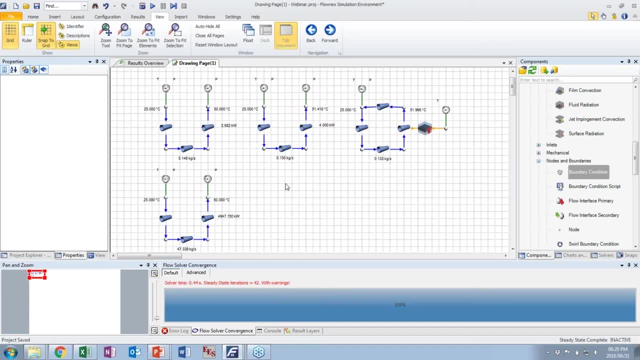 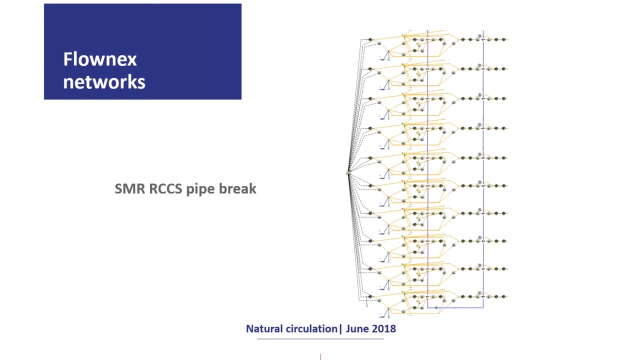 this over into a reactor which has a kind of a 2d geometry in flonix. it gets quite a lot more complicated, so let's move in that direction. i'll go back to my powerpoint slide as an example of what we've done previously. this is a small modular reactor, reactor core. 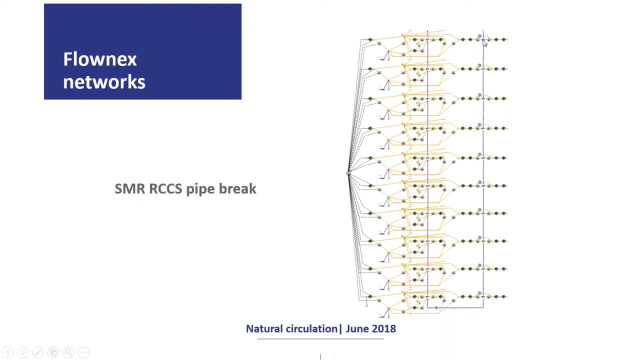 cooling system, pipe break, so we'll have flow coming down during a, during an accident case where there's no flow in the main part of the reactor, and we'll have air or some- in this case it's helium- that will cool down the outer core of the reactor. so, on a natural circulation, it will come down here, it will heat up and then 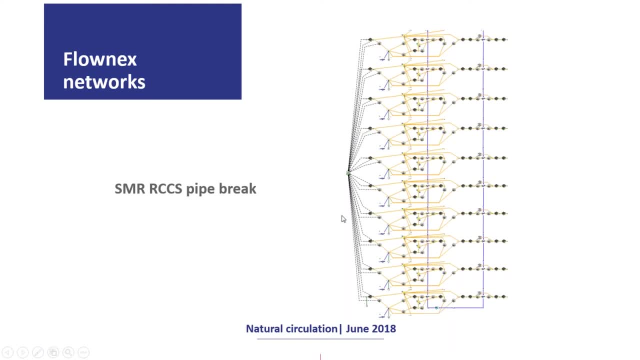 it will cool down my reactor core, also for interstate. what we've modeled here is to see if we have a pipe break from the hot side to the cold side. how will that influence this behavior? so flonix allows me, it's actually flonix allows me really some. factors. but that's another thing how to use and it actually makes for an Iranian higher pH values to influence when you produce my energy in interaction. now that is what flonix does and that's a little bit of a more in-depth explanation here. but about the sicher basic values for boiling, when you into heatYA can be, it71 is more because this in what you usually call a nuclear get and what you do if you get, talonics issue. but 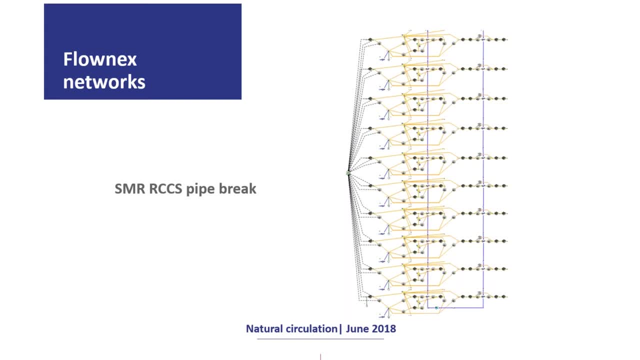 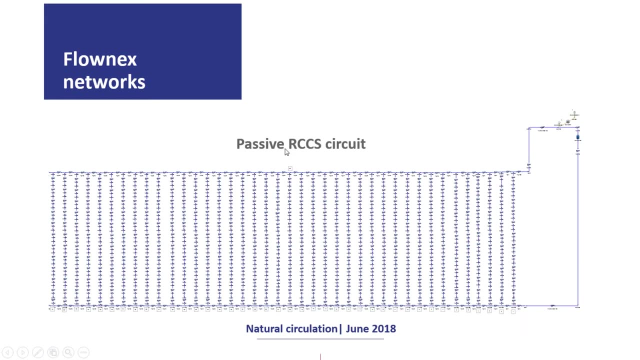 makes for a very powerful tool in order to model these accident scenarios in the nuclear field. another example is a passive reactor core cooling system circuit. so this will be water that that wraps around my reactor core. this node here and this node here is actually the same node, so 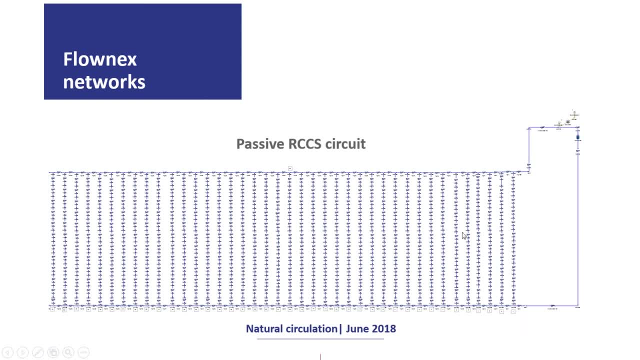 this wraps around my reactor core and i have water flowing from the bottom to the top, heat additions to all of these pipes, and that then caused a large natural circulation network with heat. they relieved to ambient conditions with the atmosphere. okay, so let's move over to reactor modeling. that's, in the end, what we are here for, and 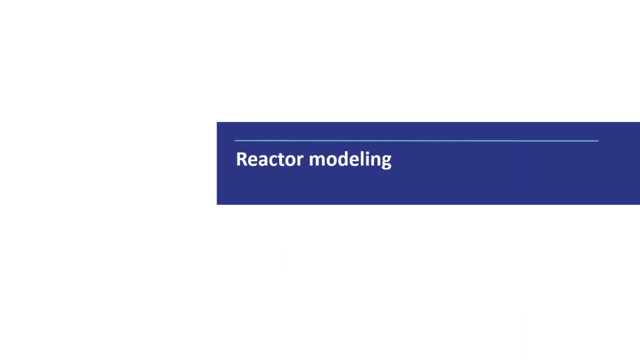 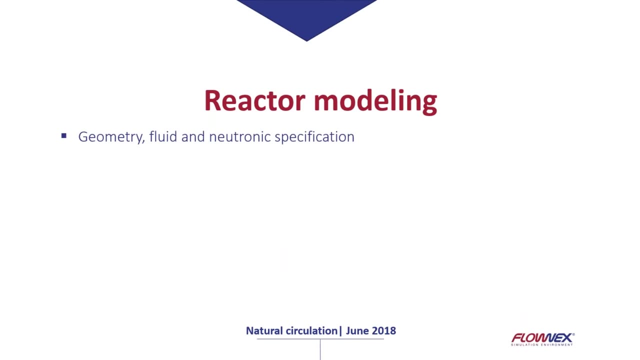 our time is almost over, so i'll try to do this as properly and as quickly as possible. in terms of flonix's reactor modeling, just a quick overview on our reactor component. it allows you to manually specify the geometry, the fluid and the neutronics within the reactor. 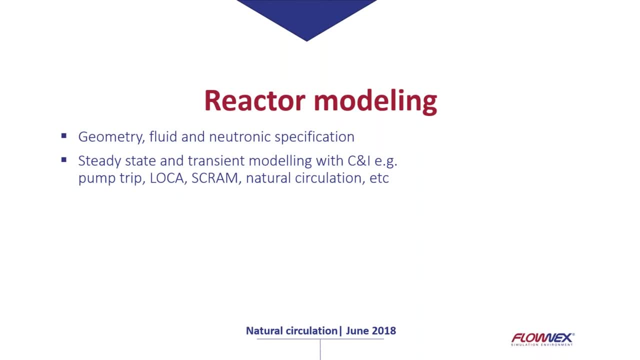 the model is set up so that we can model both steady state and transient conditions in flonix with your cni and that will be enable you to model conditions like a pump trip, a loss of coolant, accident, a scram, natural circulation, a hot air flow. that's all made possible by your real-time flow that will allow us to. 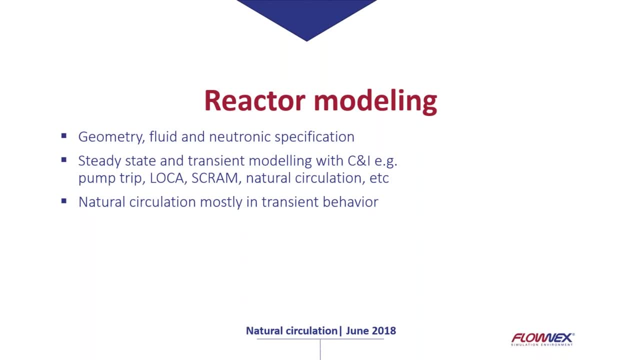 influence that flow. flow can be a little bit more complicated with a loss of coolant and the flow type will be a little bit easier. but that's all we're going to do today. so we're going to go. let's say we had a look at the flow in this example. 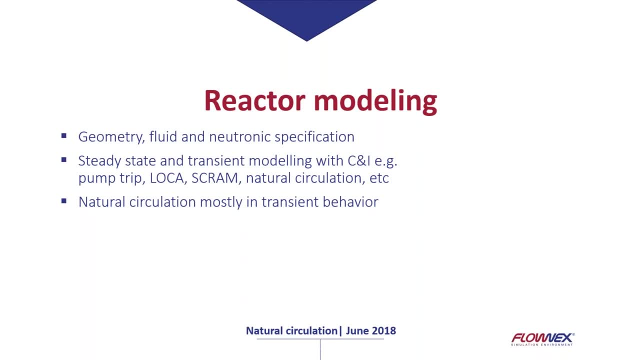 uh, up to 50 percent flow. we'll see this the way it should look here: a well-established natural convection. it's going in our reactor core in a counterclockwise direction and with that example then the flow in the middle will then stand still or within the stationary. 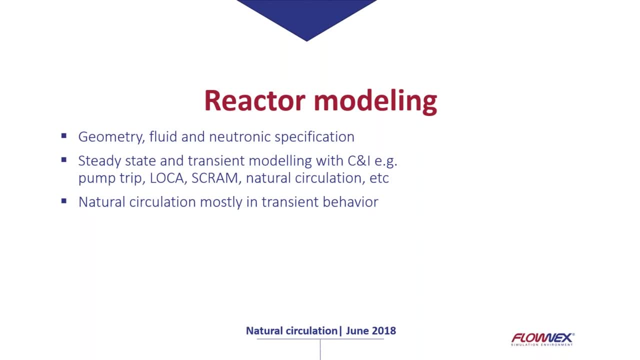 obviously in the reactor, since we still have heat generation. due to the decay heat, those fluid molecules in the middle will now start to heat up and then they will become buoyant and they will try to move to the top. so with that movement then you can see that it's going to be extremely difficult. 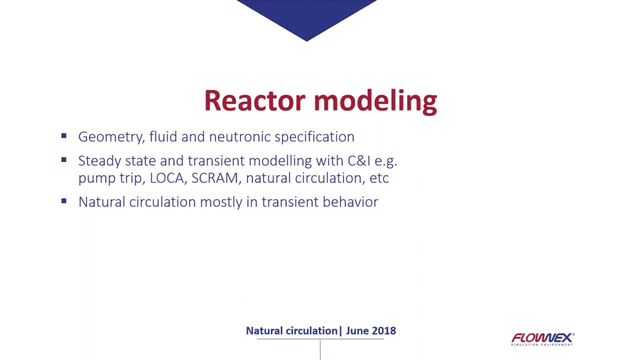 in order to achieve a steady state condition, we'll rather have flow, natural circulation flow going in various directions and in various positions, and that will change the whole time as heat is added. due to the decay heat. sometimes, in some cases, you might achieve a steady state, but it may also be that your reactor geometry and the decay heat, the heat addition, is behaving in. 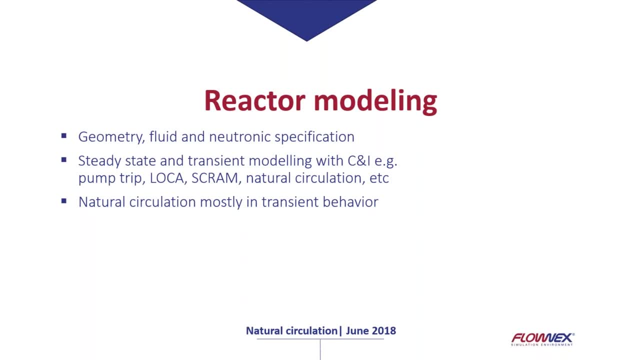 such a way that they will never be a steady state condition, and for those conditions you need to use a transient modeling in flow next. so start off with a full load condition, then simulate your accident scenario where you have your control rods drop in and the controller or your con your. 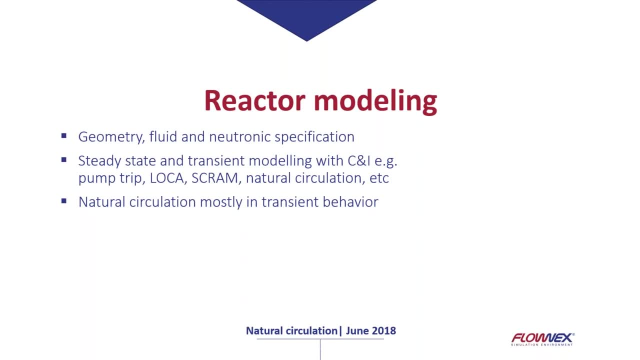 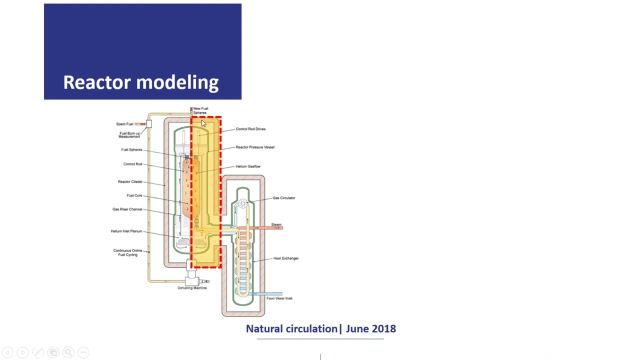 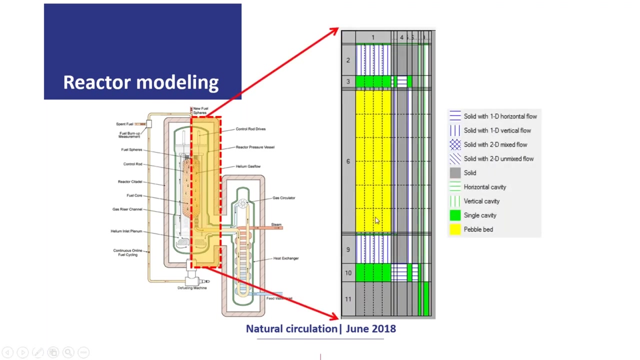 Internet controller will allow you to collaborate in aligning with the actual Dunlopp and you'll be able to cook your own food with the sample. so we need there's a little bit of areas, and then the white areas are flow paths where cooling flows will flow by. 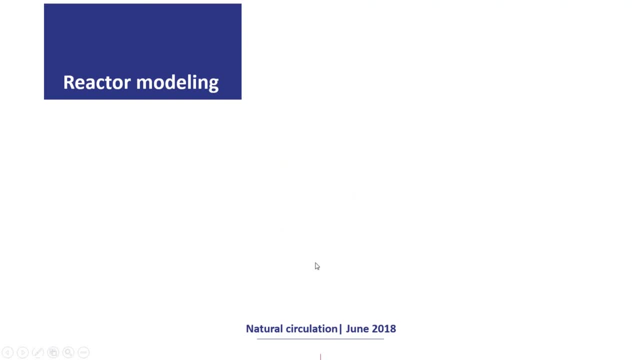 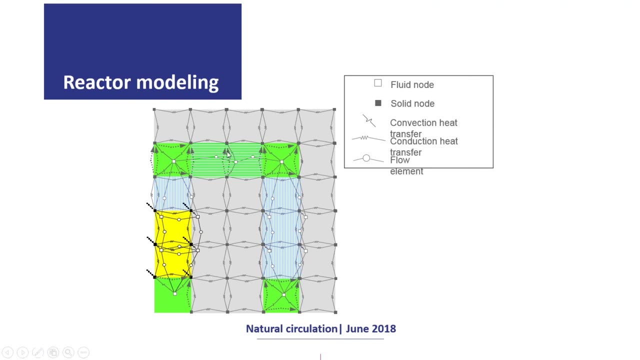 or will pass the outside of the core. that map will then be used in phonics to generate a network with convection, conduction, radiation and flow in the background and in that way then have a detailed flow next network in the background. also important to note is that the 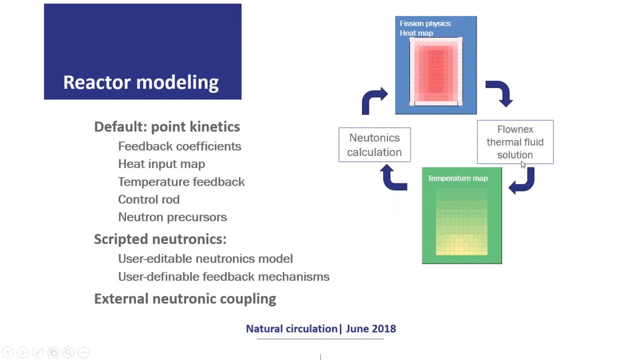 neutron, excalculation and the flow. next, thermal fluid solution works in tandem, so in in a converged solution, both these neutral to the electronics and the phonics thermal fluid solution will simultaneously come to convergence. or dependent in, yeah, dependent on each other, they will reach a converged. 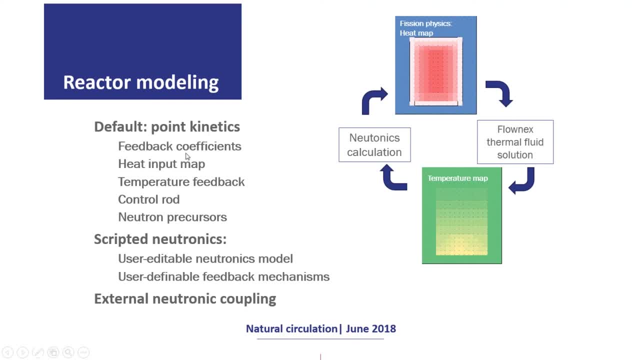 solution, so by default we have point kinetics, which includes feedback confusion and the flow. next, thermal fluid solution is a convergence solution, so by default we have point kinetics, which includes feedback confusion, coefficients, heat input map, temperature feedback control, rod behavior and neutron precursors. we also have the opportunity for you to have a user. 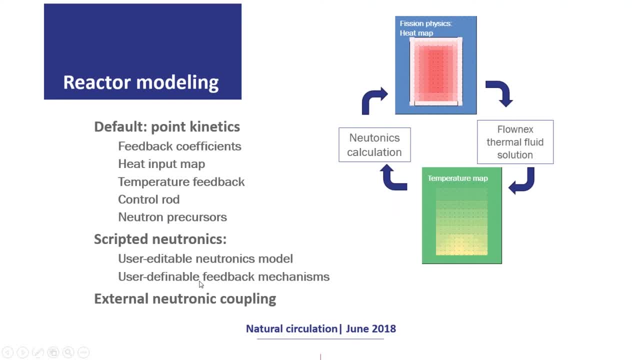 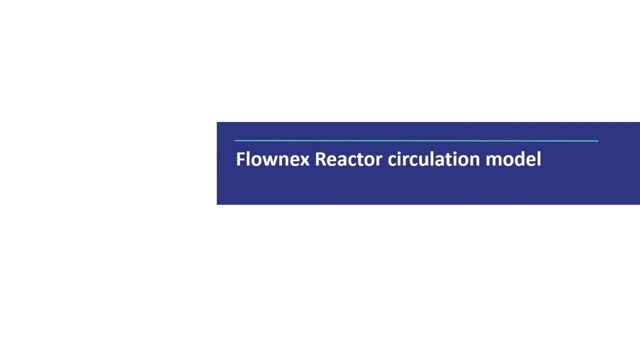 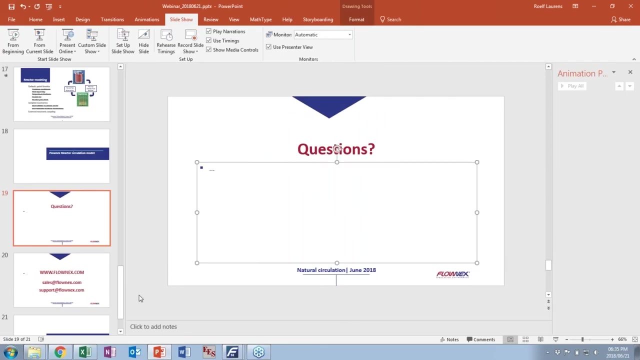 editable the electronics model script. and then a third option might be to use an external third-party software to do external neutronic coupling to the model in Flonix as a quick example that I want to show you. so I'll go to my Flonix model again. so one of the V and V cases that we have is the sauna. 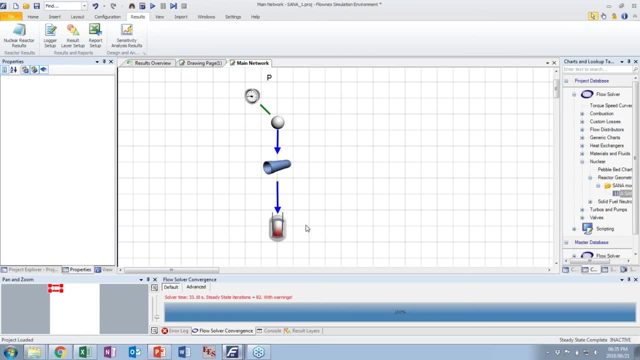 experiment which we modeled in Flonix and which we had to make sure that we achieve the same results as what they've measured on the plant during their experiments. the charts, the- the reactor charts, look something like this: so there you can see. the yellow part is. 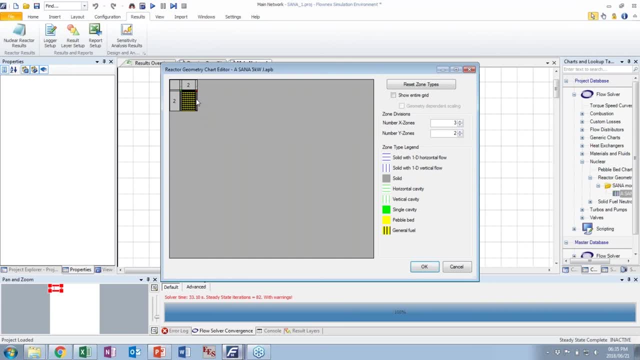 you can see the yellow part is then the pebble bed part with solids on the left and right hand side and those small red areas, and you can see they are fixed temperatures on the outside. so with this we know that the outside stays cool, the inside is hot and with that 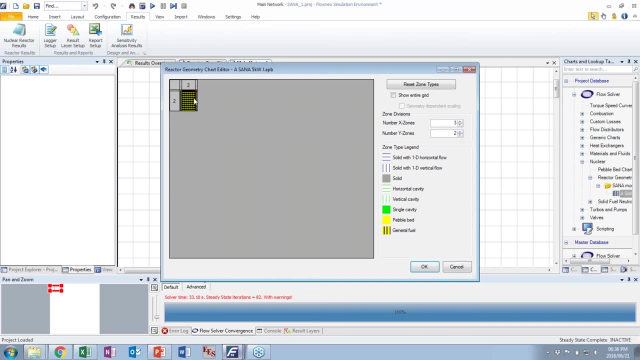 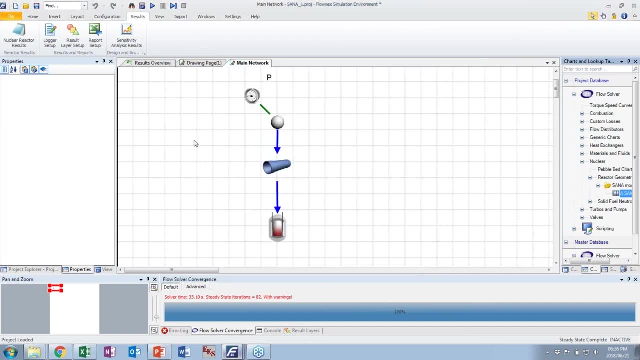 hopefully we can get natural circulation in either direction, depending on where we started off with the flow. so that is the reactor model and I solve this and in this case we achieved a steady-state solution. in order to go to the results, I will go to my results tab in Flonix and they I will see my nuclear reactor. 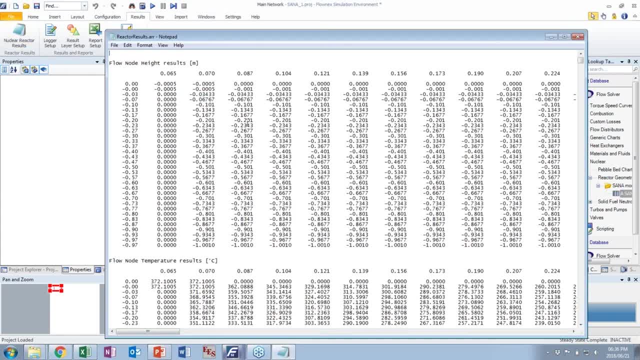 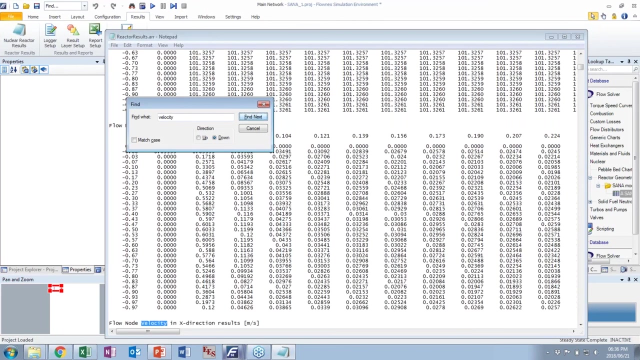 results tab and in this notepad file. all the information on that nuclear reactor component is stored in this notepad file. in order to go to my velocity results, I can simply press ctrl F to find and then say velocity and uh, there's flow node- maximum velocities. i want to go to my flow element velocities. 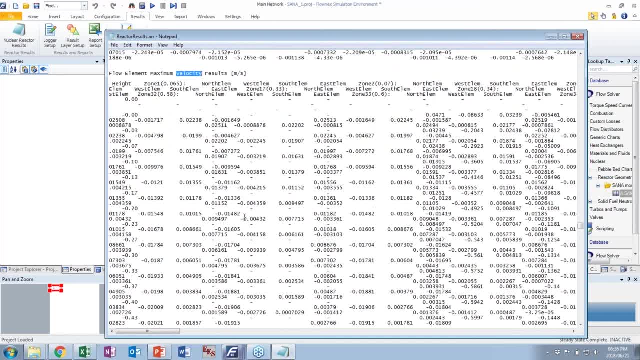 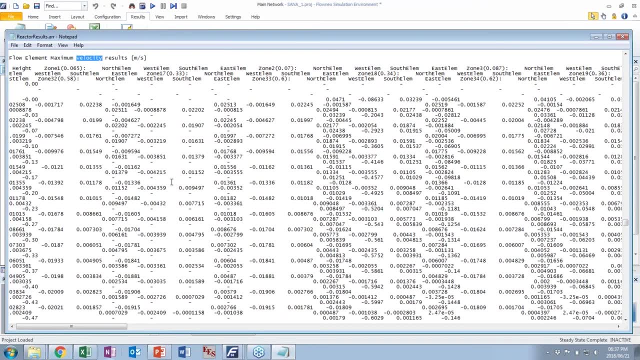 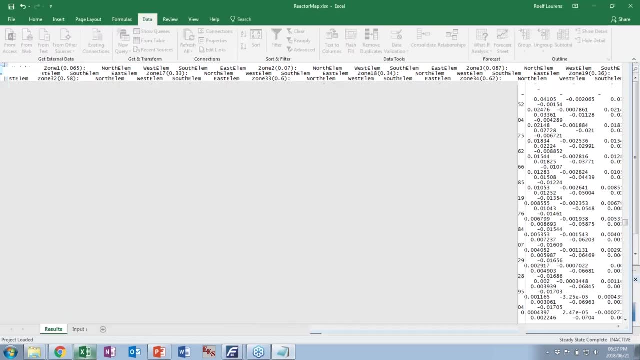 so these are on. i value just a bunch of numbers, which is quite difficult, which are quite difficult to interpret for me anyway. so what i'll do is i'll take all these values, i'll copy them and put them in excel and use excel to generate a chart such as this. so this is just in one. 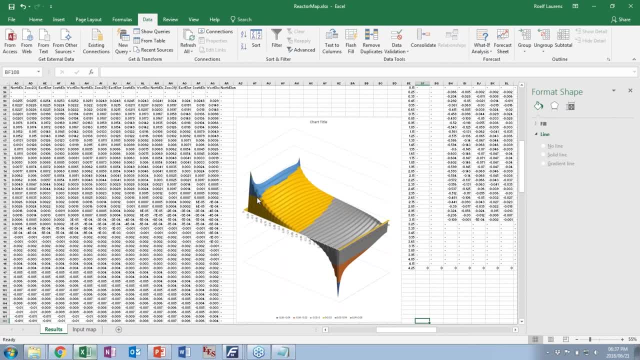 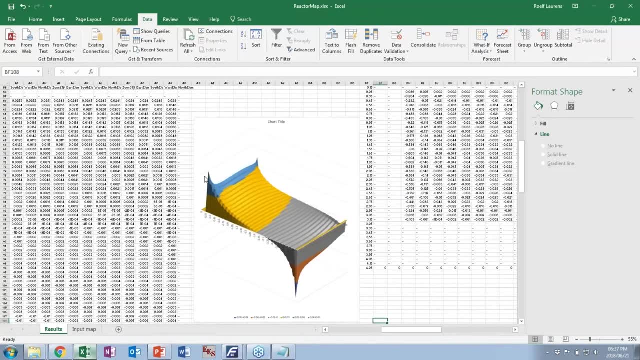 flow direction. remember, we have a two-dimensional grid in flow next, so this will be in one direction. i will have flow in another direction as well, and then these values will show me, for this experiment, how we, throughout the reactor, how we have different zones of flow. so here we. 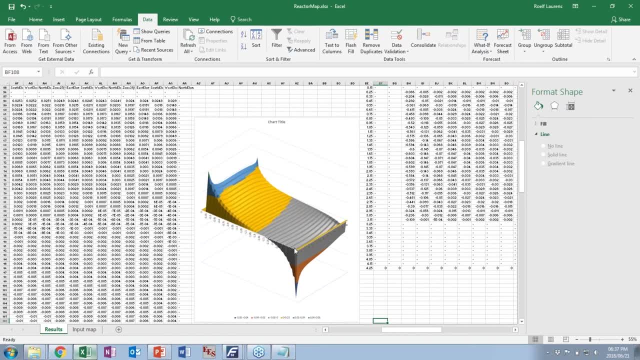 have positive flow and at the here we will have flow in another direction, and then we will have flow in another direction, and then we will have flow in another direction and we'll also have some flow profile going through the reactor. so with this then i can- it's a very good way of visualization, of visualizing my natural circulation flow within my reactor. 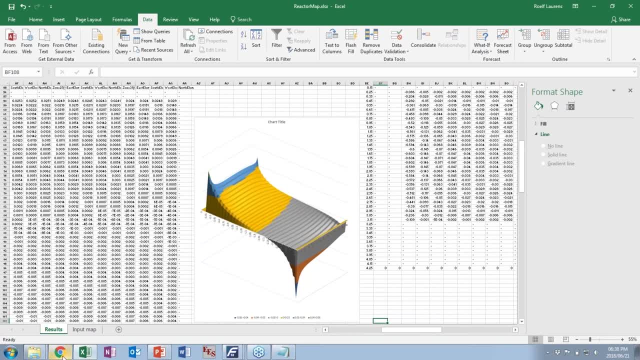 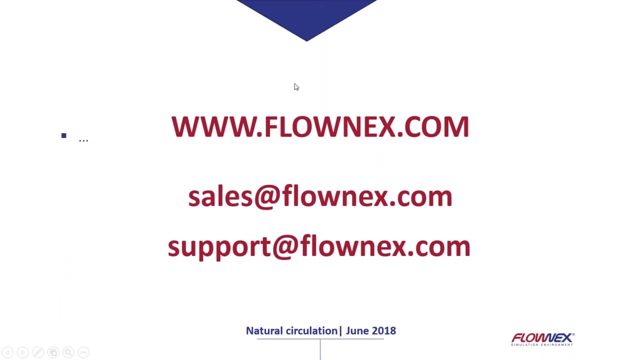 unfortunately, that's about all we have time for that. i had to rush a little bit through the last part, so please send me an email. you can just get the email address there on your screen, so that will be our email address. is? that's the website. so if you are new to flonix and you would like to find out more about,